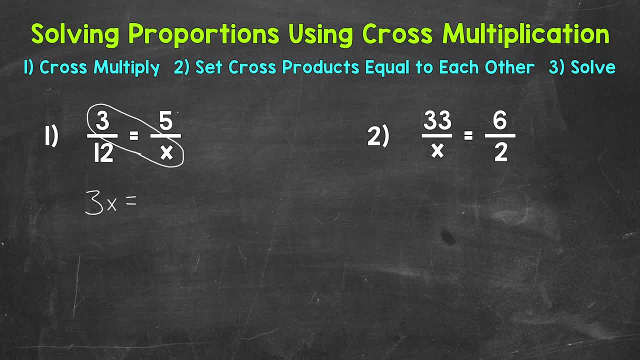 We can bring our equal sign straight down and then we have 12.. Now I'm going to use a dot to represent multiplication. That way there isn't any confusion between x's that are variables and then x's that are multiplication signs. 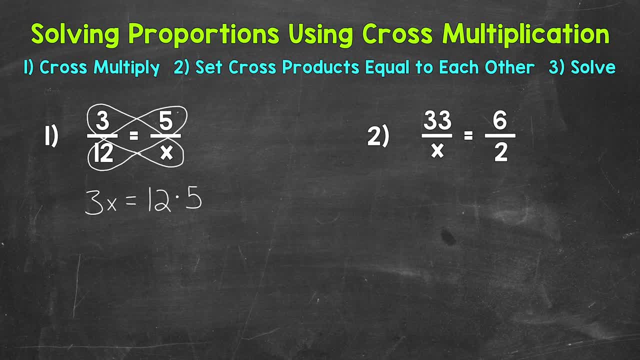 Now we can do 12 times 5.. Let's bring our 3x down. Well, 12 times 5 equals 60. We have: 3x equals 60. Now we have a one-step equation That we can solve to figure out what x equals. 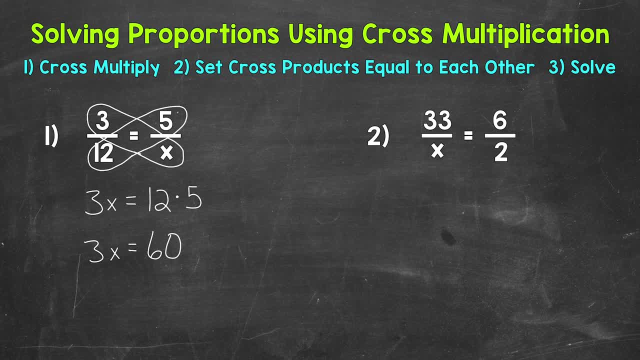 So we need to isolate that variable of x. We do that by dividing both sides by 3.. So 3x divided by 3, and 60 divided by 3.. 3x divided by 3 gives us x, and then 60 divided by 3 gives us 20.. 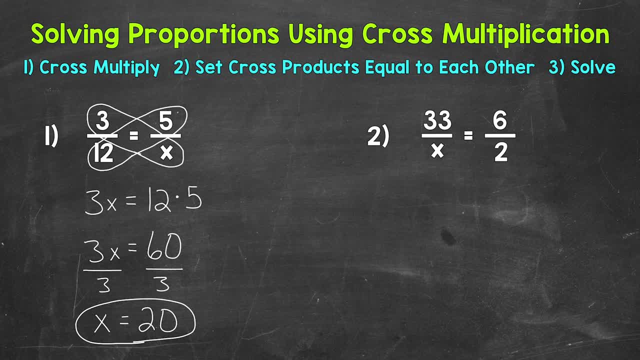 x equals 20.. x equals 20.. Now we are just slowly getting more inside our system and so trying to figure out which side of the cross-product works against what is on the x quadrant Once you do calculate the cross-partition. 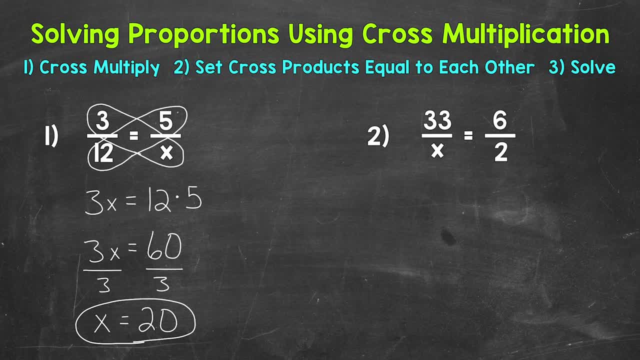 you will visit that terug. Let's go back to this English class a little bit. and now that we are in class, Webinariał equals 6 to 2.. We'll start by cross-multiplying, so multiplying diagonally First, we'll do 33. 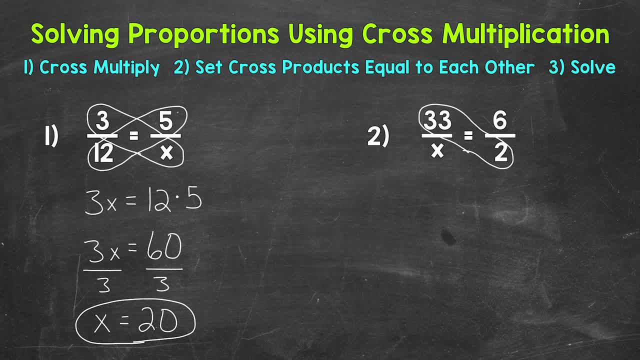 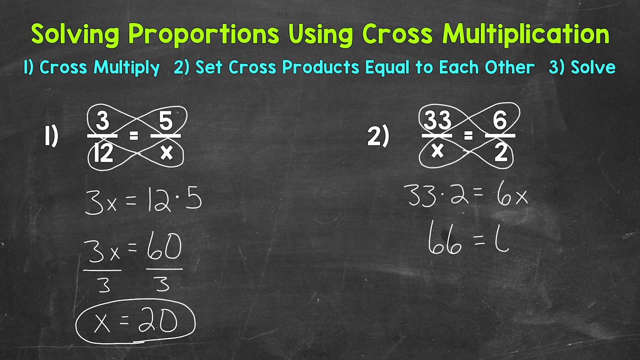 times 2.. So we have 33 times 2.. Bring our equal sign down and then we have x times 6,, which we can write as 6x. Next we can do 33 times 2.. That gives us 66.. Bring our equal sign and 6x. 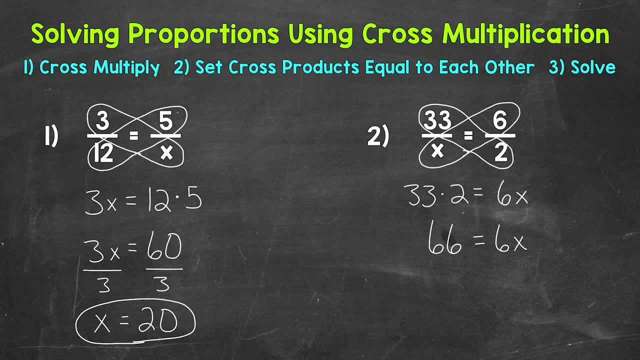 down. Now we have a one-step equation that we can solve. in order to figure out what x equals, We need to isolate that variable of x, and we can do that by dividing both sides by 6.. 6x divided by 6 will isolate that. 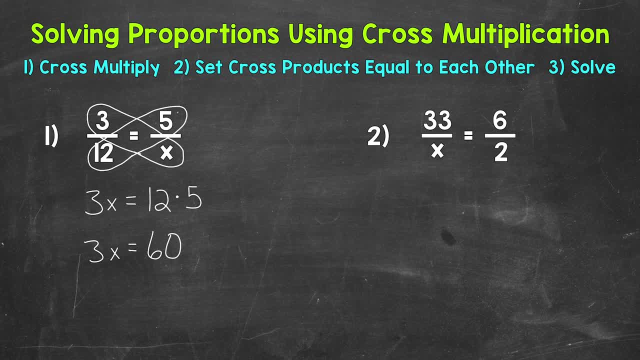 So we need to isolate that variable of x. We do that by dividing both sides by 3.. So 3x divided by 3, and 60 divided by 3.. 3x divided by 3 gives us x, and then 60 divided by 3 gives us 20.. 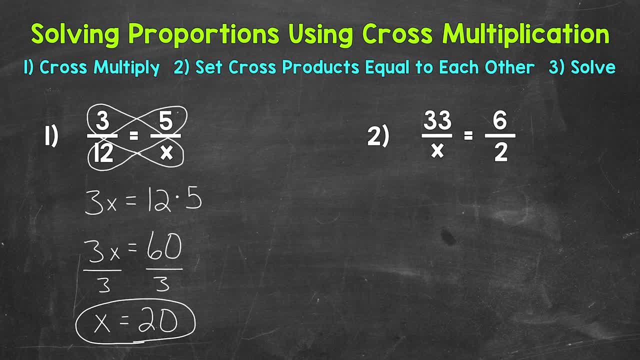 x equals 20.. x equals 20.. And now we can solve to per Camille, Remember to add this to your calculator. Another thing I do want to mention about using cross multiplication to solve proportions. Don't get two held up. on what numbers to multiply first? 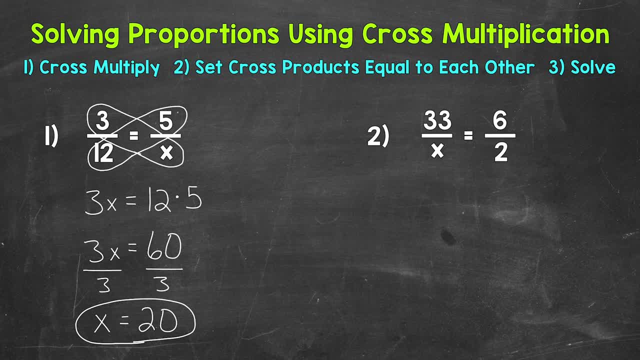 or which diagonal you should put on which side of the equal sign. It will all work out the same either way. Just make sure to multiply diagonally and have the equal sign in between your cross products. 3 to x equals 6 to 2.. 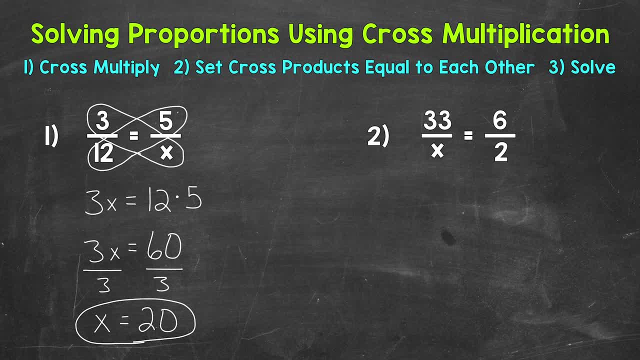 We'll start by cross multiplying, so multiplying diagonally. First we'll do 33 times 2.. So we have 33 times 2.. Bring our equal sign down, And then we have x times 6, which we can write as 6x. 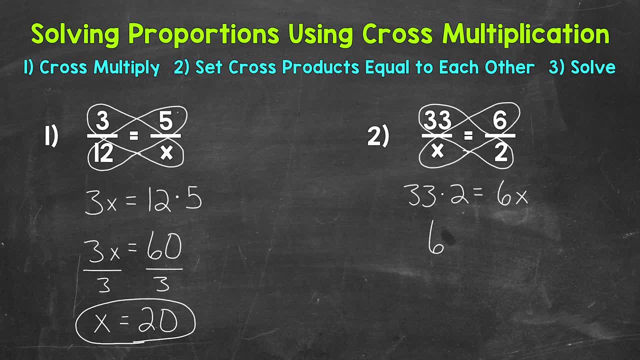 Next, we can do 33 times 2. That gives us 66.. Bring our equal sign and 6x down. Now we have a one-step equation that we can solve. in order to figure out what x equals, We need to isolate that variable of x, and we can do that by dividing both sides by 6.. 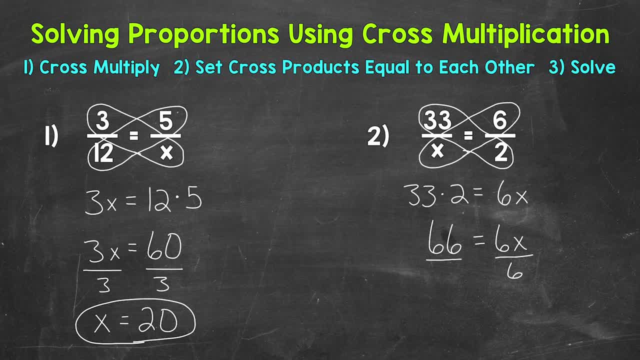 6x divided by 6 will isolate that x. And then we also need to do 66 divided by 6. 6x divided by 6. Again isolates that variable. So x equals, and then 66 divided by 6 gives us 11.. 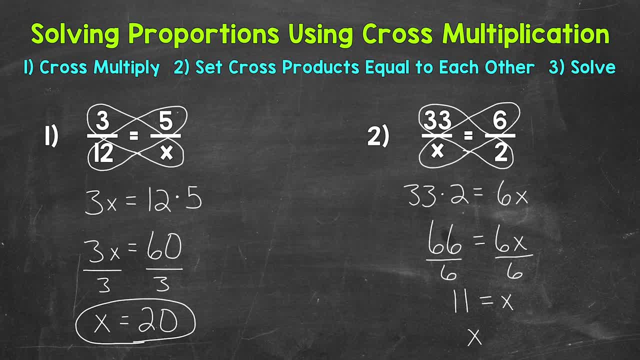 So x equals 11.. And we can rewrite that as x equals 11.. So there you have it. There's how you solve a proportion using cross multiplication. Cross multiply, set the cross products equal to each other and solve. I hope that helped. 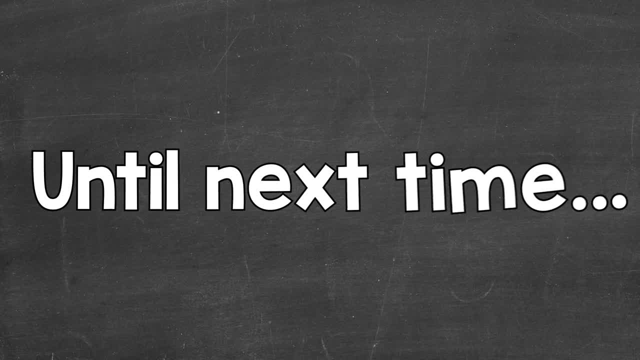 Thanks so much for watching. Until next time, peace.